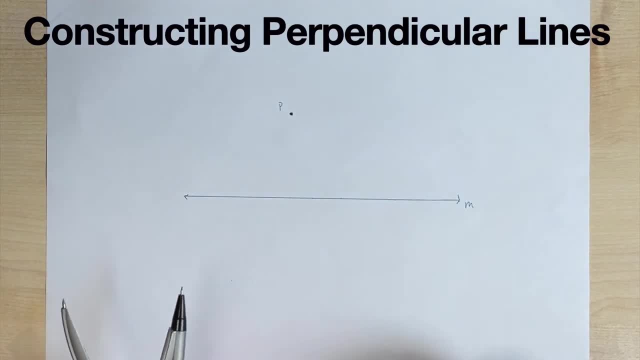 line that goes through point P and is perpendicular to line M. Now in this video we're not going to do a perpendicular bisector. We'll do another video where we look at how to construct a perpendicular bisector. So for this one we're just doing perpendicular lines, So we're not necessarily 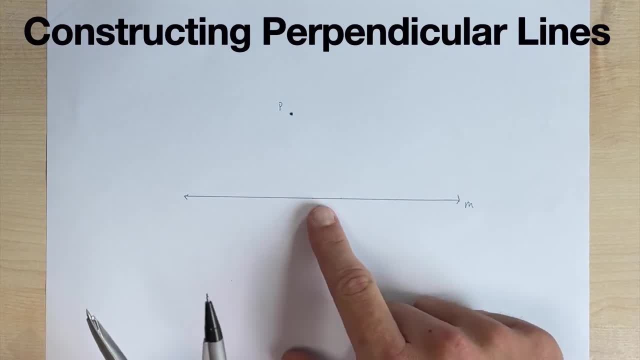 worried about if our perpendicular line goes through the middle of our line M, because, once again, this is not a bisector, This is simply just a perpendicular line. I'll link the video to the perpendicular bisector below. All right, so what we're going to do to start off is we're going to: 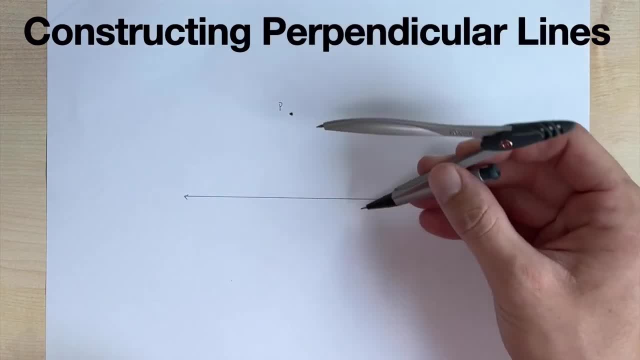 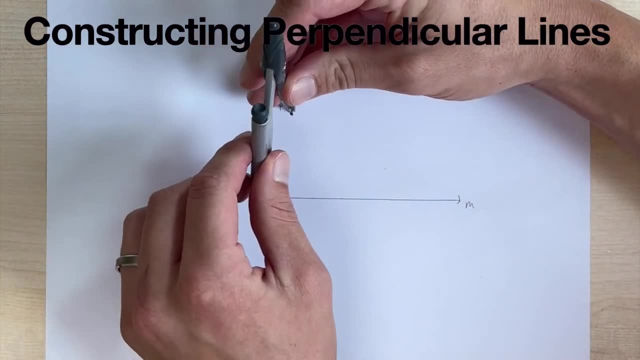 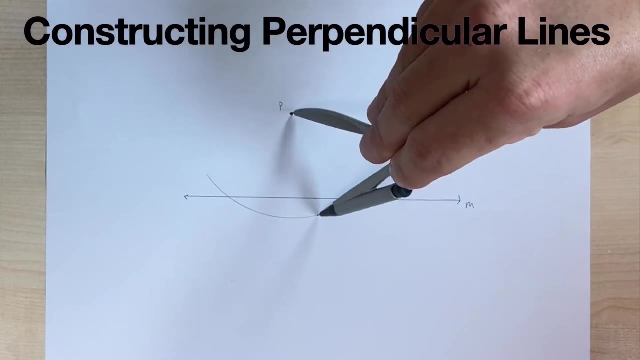 put the needle of our compass on point P and we are just going to make an arc on line M that intersects line M twice. So we'll put the needle at P and we're going to draw an arc and just make sure this arc intersects two places on our line. Okay, so now we have our arc and we have a couple. 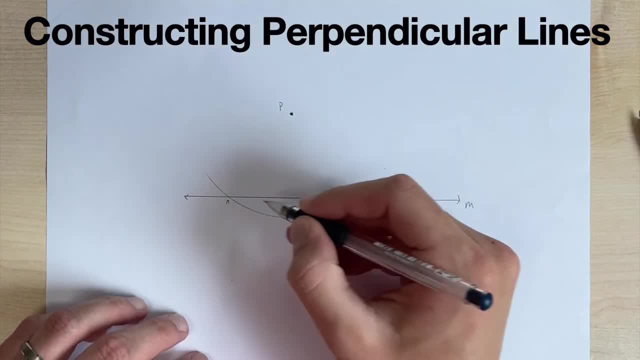 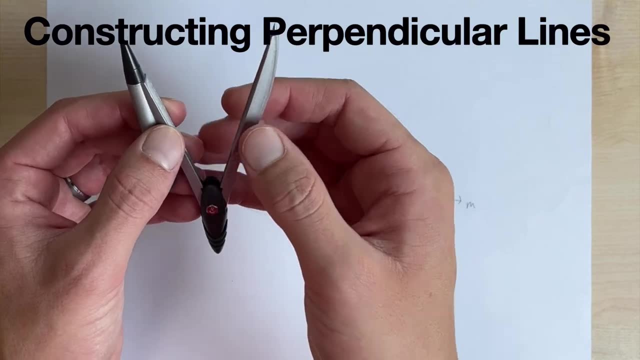 intersections here. Let's label these intersections A and B, All right. so now what we're going to do, it doesn't matter how, how your compass is at this point. If you want to close it up a little bit, that's fine, but what we are going to do is put 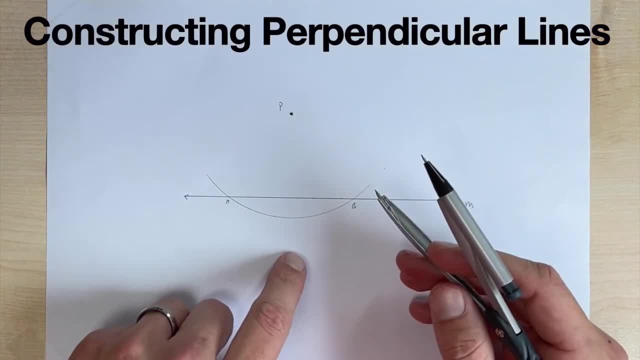 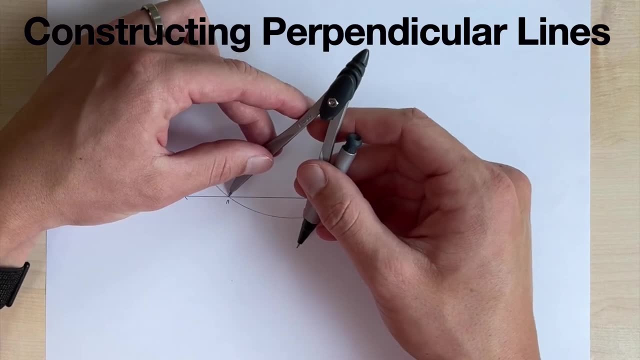 the needle at A and we're going to make an arc down here, and then we'll keep the compass open. the same amount. We'll put the needle at B and we'll make another arc down here as well. So right now we're going to put the needle at this intersection where we have A and we're just. 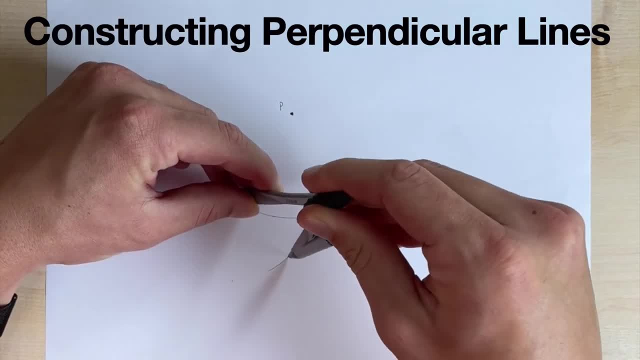 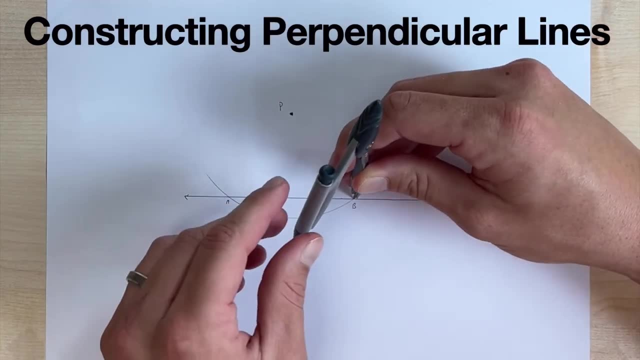 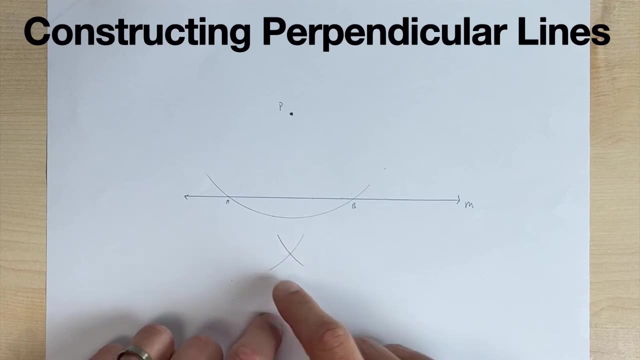 going to make an arc down here, Just like this. Okay, now keep the compass open. the same amount. Now move the needle to the intersection that we have labeled B, and we're going to make an arc down here. All right, so now, notice, we have an intersection down here. We could call this intersection C, and now we're going to. 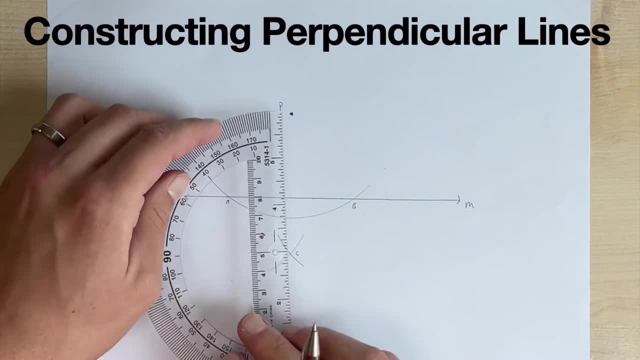 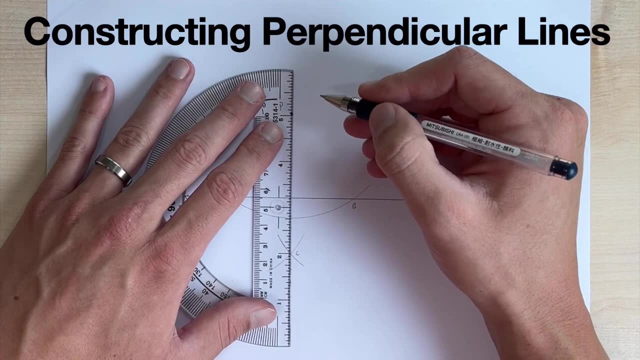 take our straight edge and we're just going to draw a line that goes through our intersection and our point P. Okay, so those should line up, Line up right on top of each other, and we're going to draw our perpendicular line, just like that. 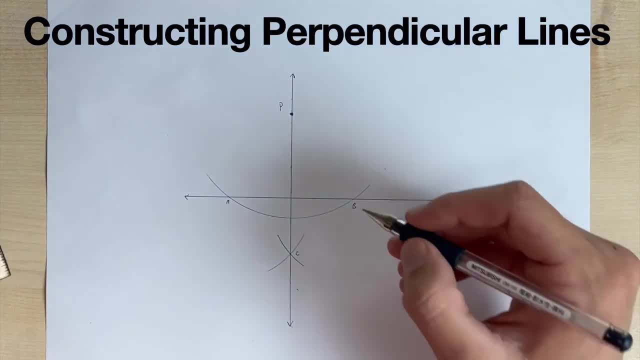 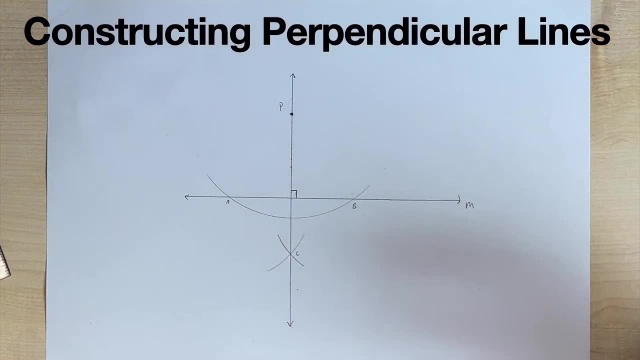 Okay, and so now, to indicate that this is a perpendicular line, we can draw our 90 degree or our right angle box right there and we have constructed perpendicular lines. So we could say: that line, we call this line PC. All right, that would be our vertical line PC. and we could say: 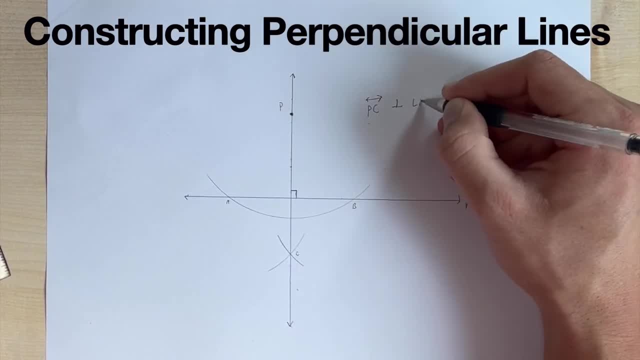 it is perpendicular to, and we're going to draw a line that goes through our intersection and we're going to call this line M, and that's how you construct perpendicular lines. 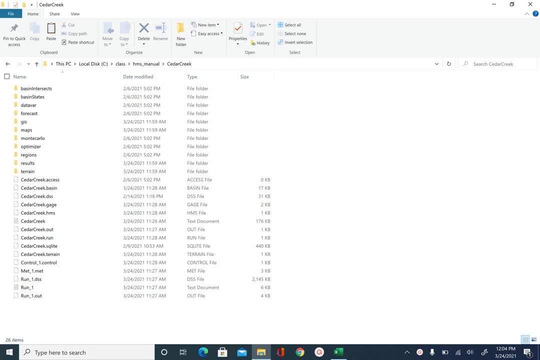 In this unit, we are going to learn how to manually calibrate a HEC-HMS model. In order to finish this unit, you need to have a HEC-HMS model with observed hydrograph, and this is something we have done earlier in module 7.. So what I have? 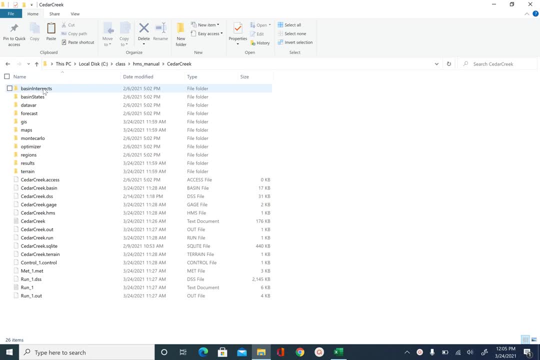 done is I have just copied that folder that has the Cedar Creek model. So folder with Cedar Creek model will have all these files and folders. So once you copy that you should be able to start. and even if you don't have it, it is. 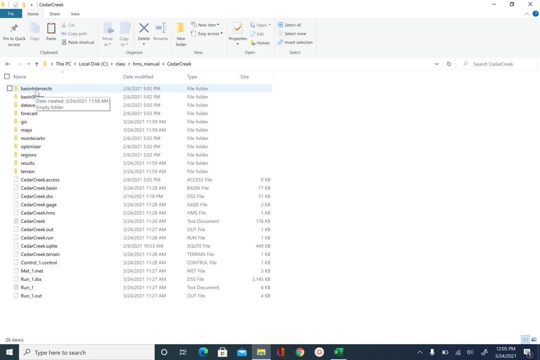 provided with this unit, so you should be able to download and copy it in your folder. I have named this folder as HMS underscore manual because in another unit we are going to learn how to calibrate a HEC-HMS model using the optimization of HEC-HMS model.